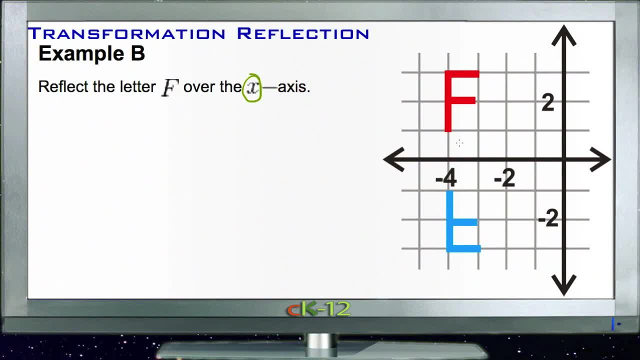 x coordinate is going to stay the same and it's the y coordinate that's going to change. So if we had, say the bottom point of our f letter here at negative 4, 3,, negative 4, 1, then its new location would be the same x value, so still negative 4, but now the 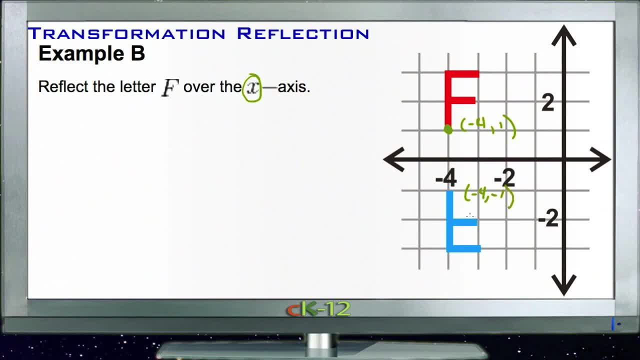 opposite sign on the y value: negative 1.. Yeah, And if our top point up here was at negative 4, 1,, 2, 3, then our bottom coordinate, or the corresponding one, would be at negative 4, negative 3.. 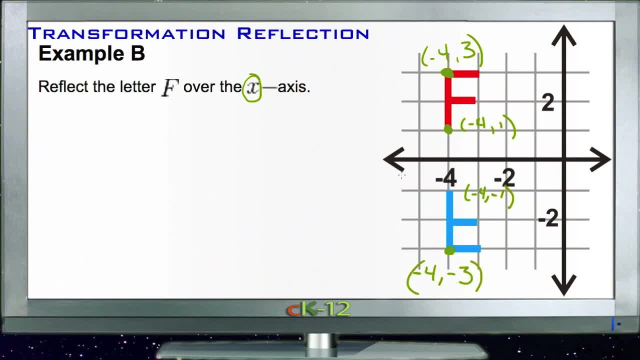 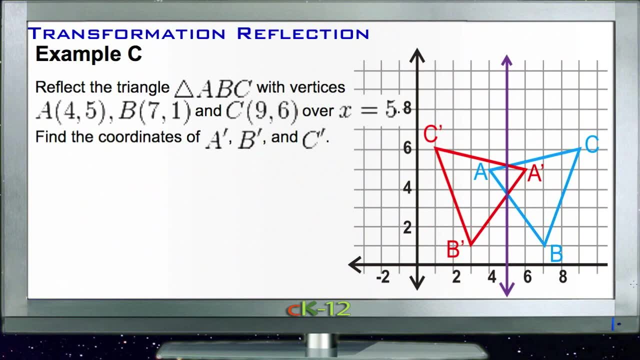 x coordinate stays the same, y coordinate changes because we're reflecting over the x-axis, Cool. And then finally, example C Reflect the triangle ABC that has the vertices a, 4, 5.. So 1,, 2,, 3,, 4, 5, right here, And b 7, 1, right here, And c 9, 6 over the line x, e right. 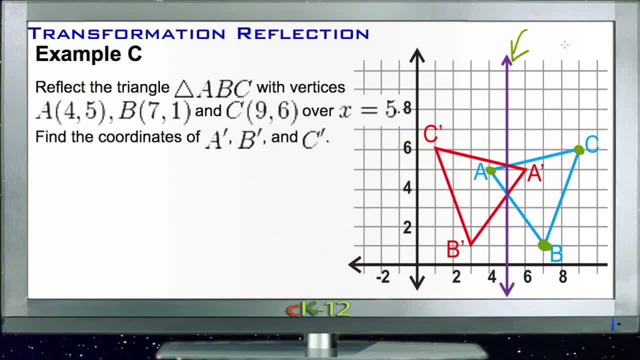 equals 5.. So that's this purple line right here. So if we're going to reflect it over the line, remember each point. now we're reflecting over an x, I'm sorry, over a y line, so our y line, our y coordinates are going to stay the same and our x coordinates 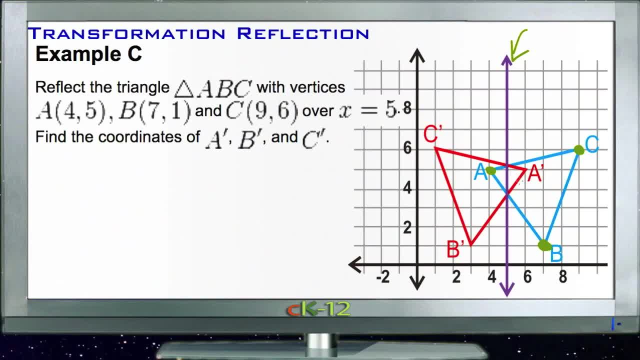 are going to be the ones that change right. So we're going to go from with our a coordinate right here, which starts out at 4, or one point away from the line on the left. when it reflects, it's going to be one point away from the line on the right, but the y coordinate 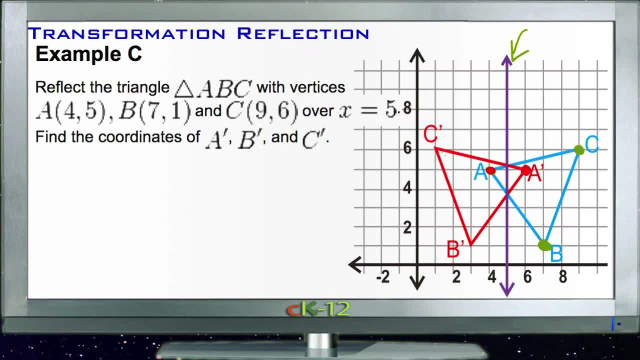 is going to stay the same For c. c starts off with 1, 2,, 3, 4, 1,, 2,, 3, 4 points away from the line to the right, so its reflection is going to be 1,, 2,, 3,, 4 points away from. 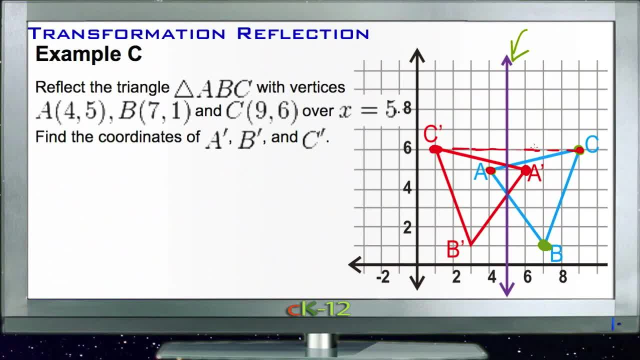 the line to the left and the y coordinate stays the same. The b point starts off 1,, 2,, 3, 4,. 1,, 2,, 3, 4 points away from the line to the right of the line, so its reflection.